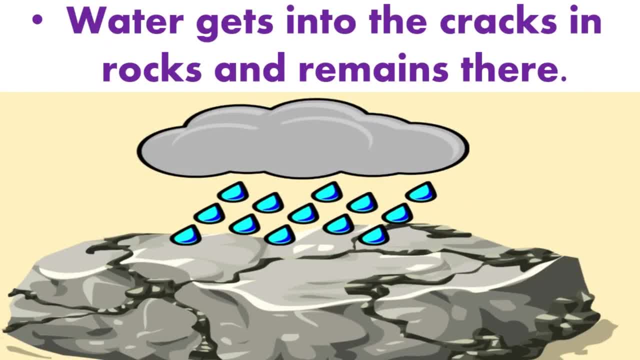 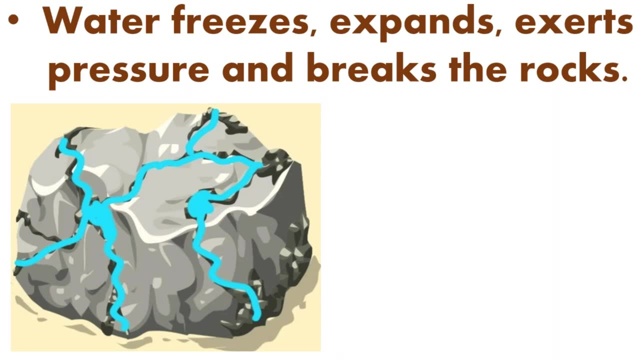 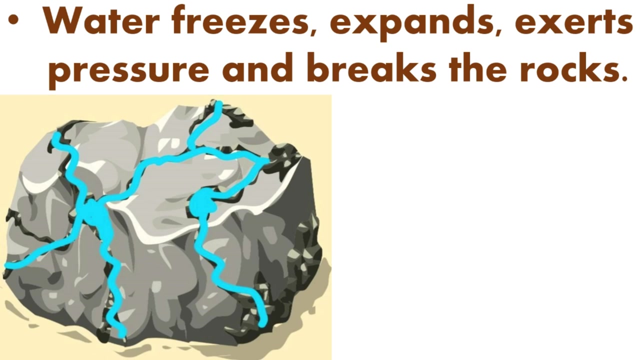 So you all know that soil is formed from rocks. So when it rains, water gets into the cracks in the rocks and remains there. And when weather changes, the water present in the rock freezes expands and it exerts pressure And because of this pressure, the big rocks start to break down into smaller rocks. 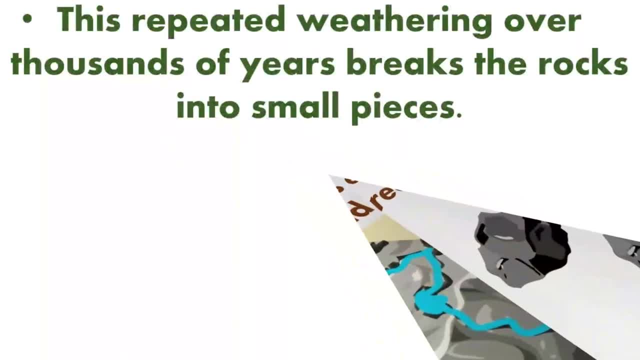 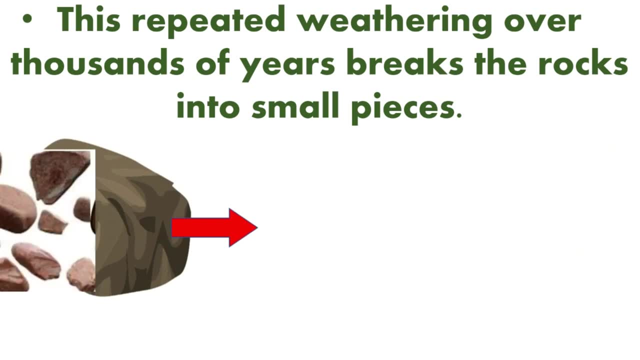 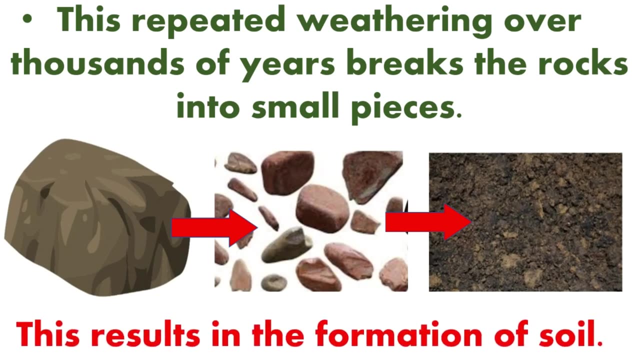 So when weather changes, the water present in the rock freezes expands and it exerts pressure. This repeated weathering over thousands of years breaks the rocks into small pieces And this results in the formation of soil. So formation of soil from rock is not a very quick process. 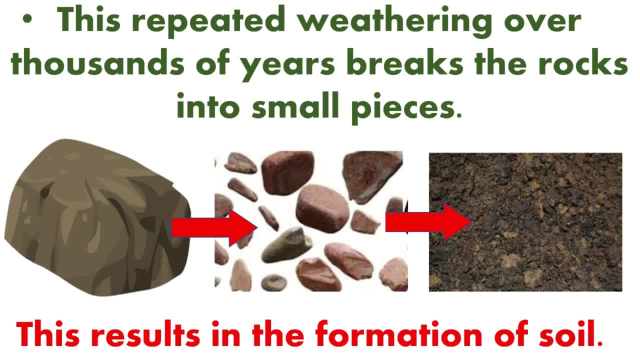 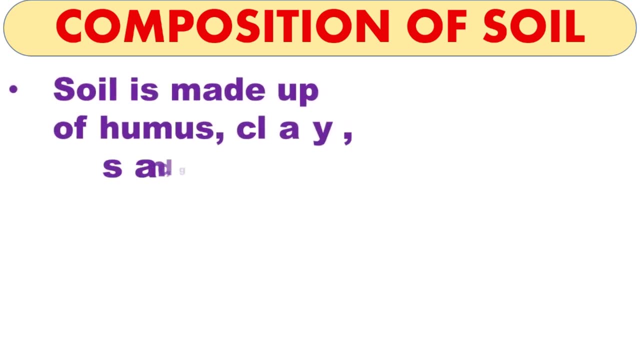 Or you will say it takes few months or few years. No, it takes millions of years For rocks to change into soil. And next is composition of soil. Soil contains many things. Soil is made up of humus, clay, sand, gravel and minerals. 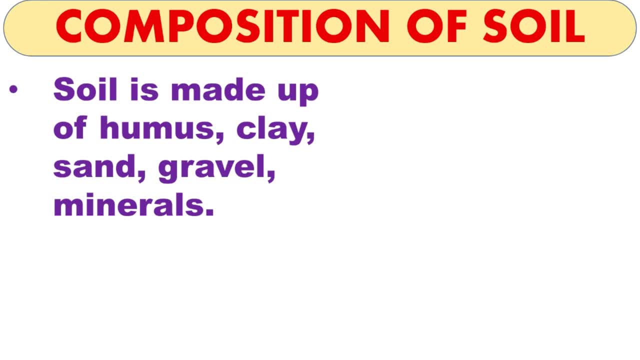 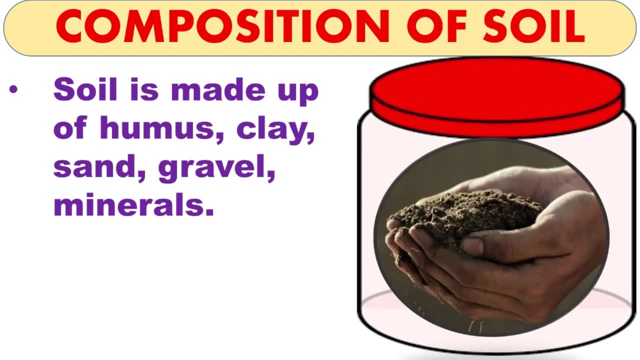 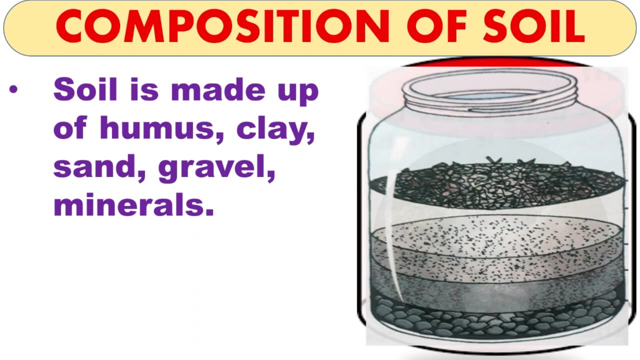 For this you can also do an activity. So take a glass jar, dig out some soil from the garden and put it in the jar And then pour some water in the jar. After some times you will see several layers in the jar, as you can see in this picture. 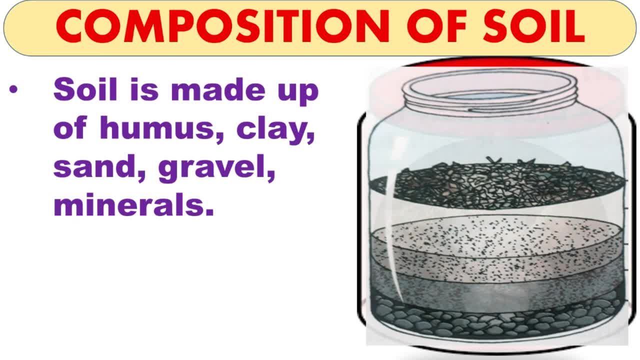 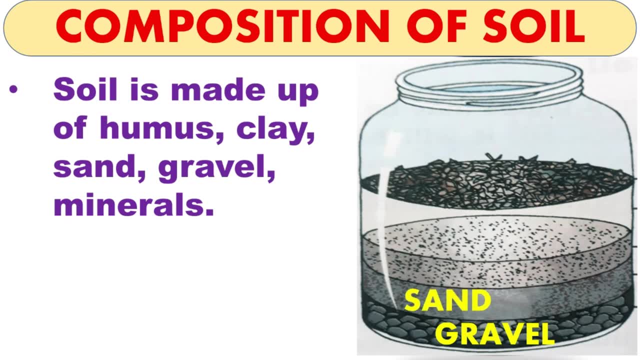 The bottom layer is made up of small stones called gravel. Above this is the layer of sand. The sand particles are much smaller than gravel. Next is the layer of very small fine particles, And that is clay. The clay particles are so small that you cannot see them separately. 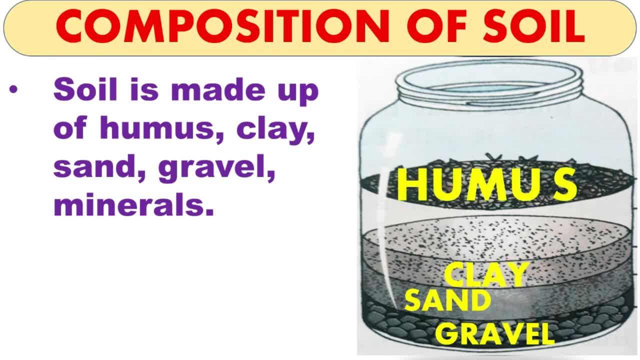 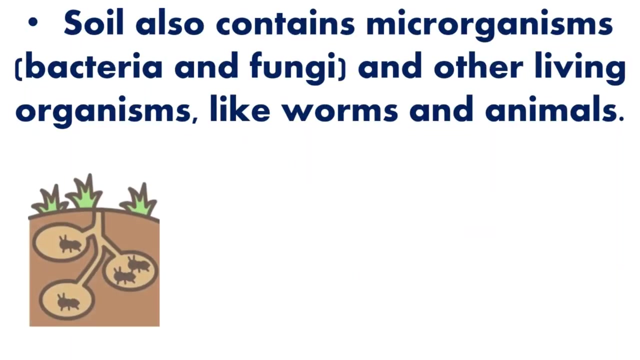 And on the top you will see the humus. What is humus? When plants and animals die, they decompose or break down and get mixed with the soil, Forming humus. Soil also contains air and water. Soil also contains microorganisms like bacteria or fungi. 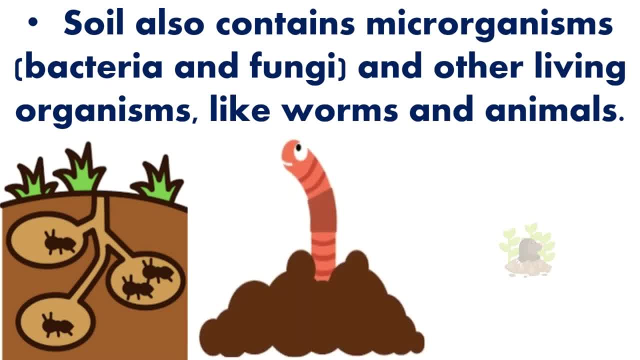 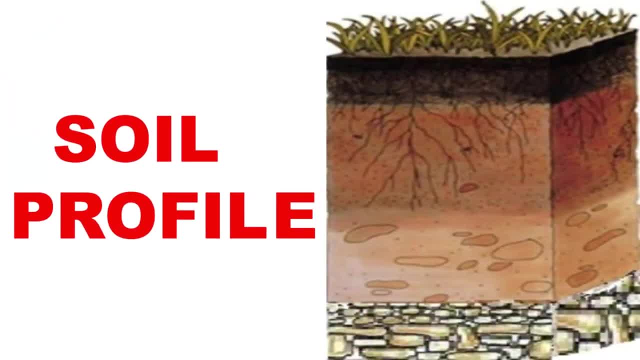 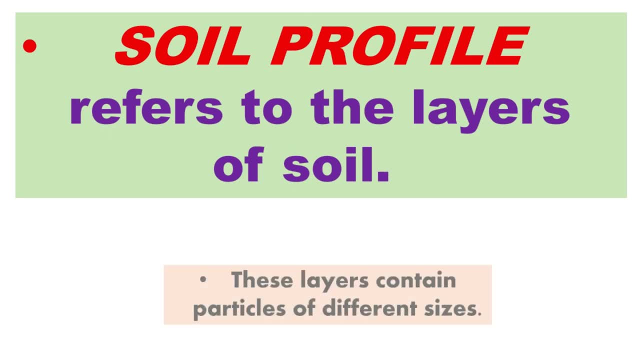 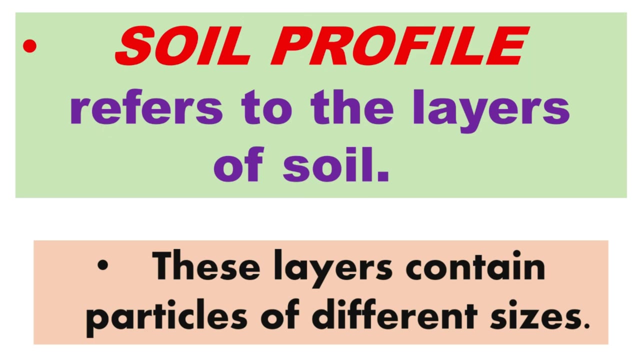 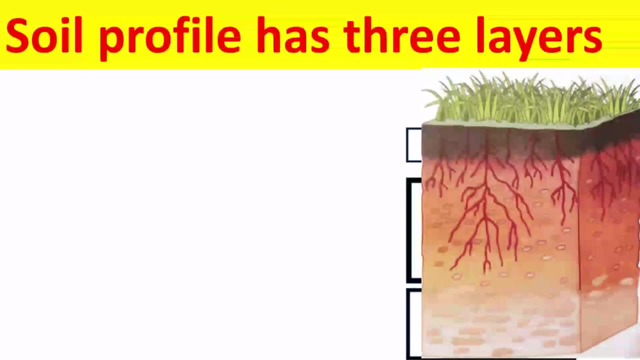 And other living organisms too, like worms and animals. So next is soil profile. Soil profile refers to the layers of soil, And these layers contain particles of different sizes. Particles can be small rocks, stones, pebbles, etc. Soil profile has mainly three layers. 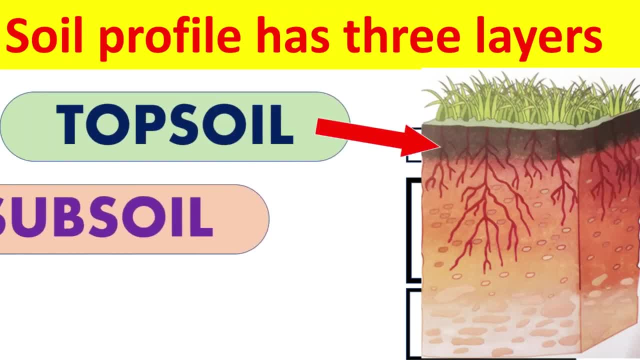 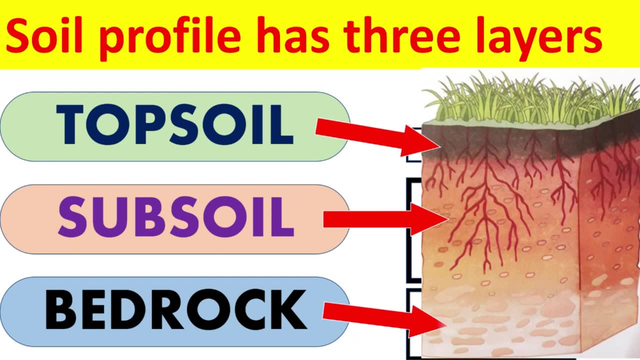 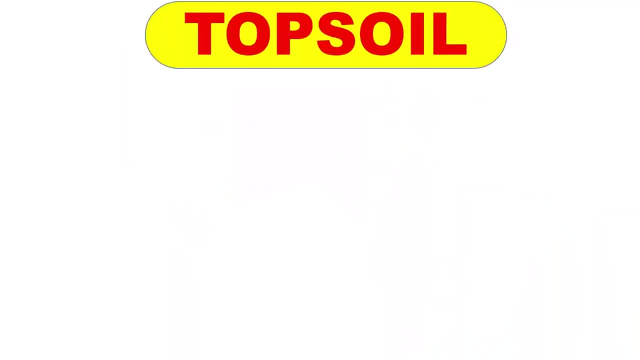 The uppermost layer is the topsoil, The middle layer is the subsoil And the bottom most layer is the bad rock. So now let us have a look on these layers in detail. So first we will talk about topsoil. 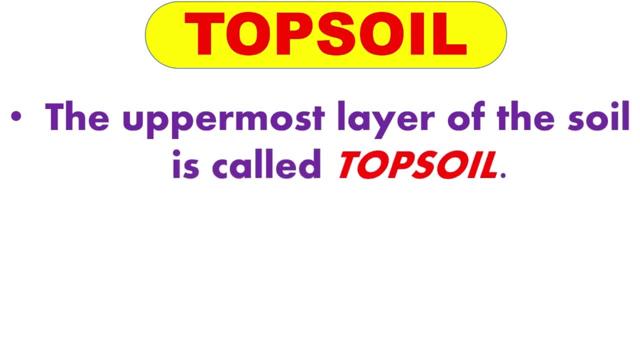 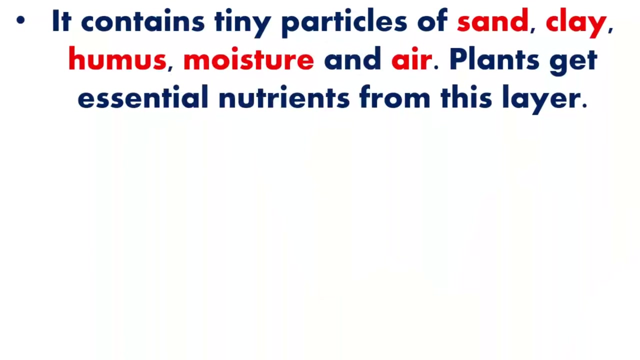 The uppermost layer of the soil is called topsoil. Almost all agricultural activities are done in this layer. Farmers sow their seeds in this layer And in this layer mostly, roots of the plants spread out and grow. The uppermost layer of the soil is the topsoil. 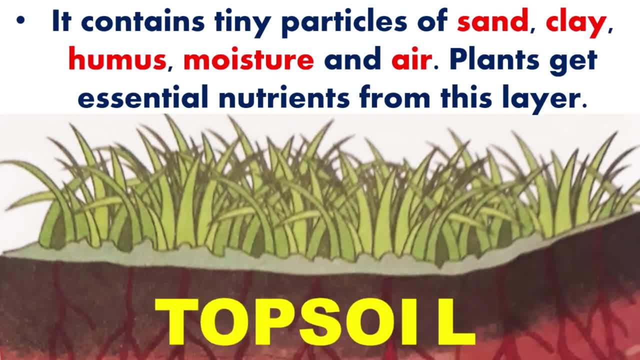 And topsoil contain many particles of sand, clay, humus, moisture and air And plants get essential nutrients from this layer And on this layer there is lot of humus in the soil And the plant grows very well in this layer. 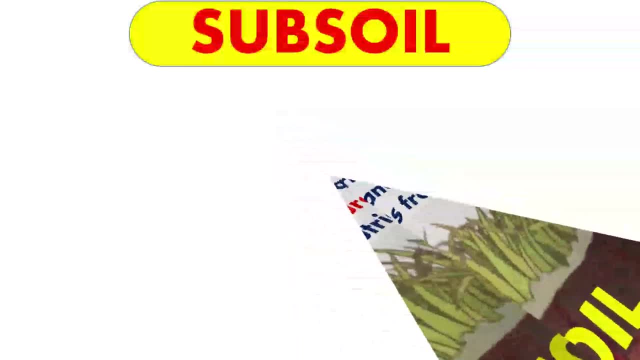 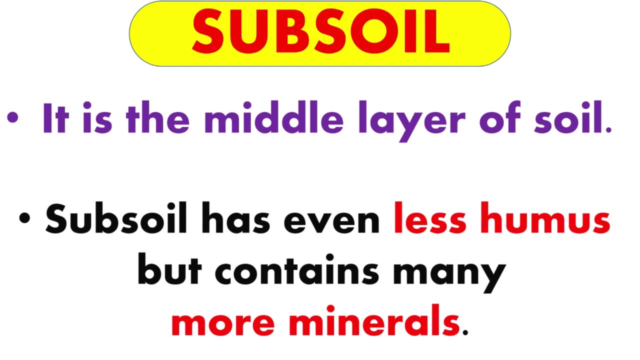 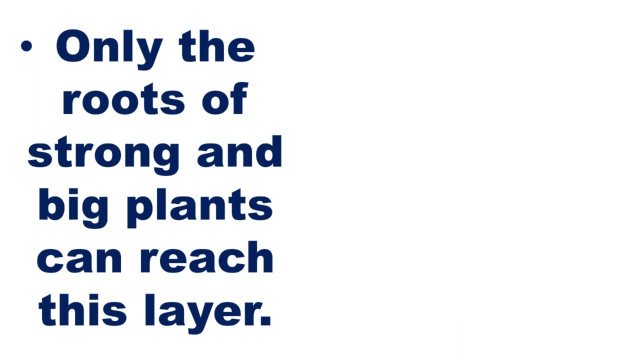 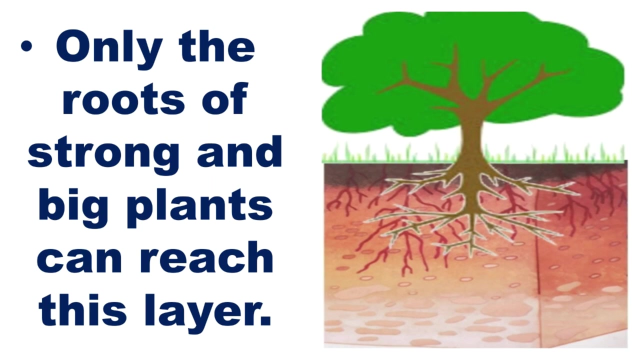 So next is subsoil. It is the middle layer of the soil. Subsoil has even less humus than topsoil, But contains many more minerals. And subsoil is hard and less porous than topsoil, And because of this only the roots of strong and big plants can reach this layer. 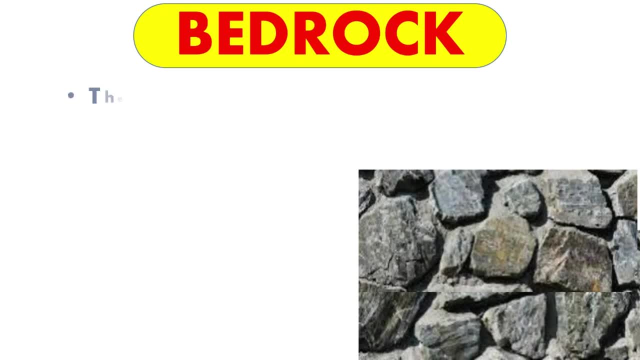 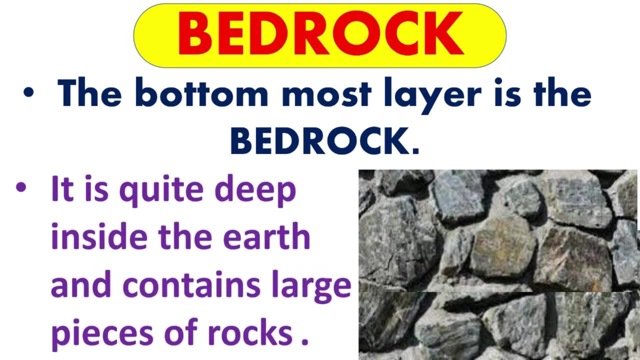 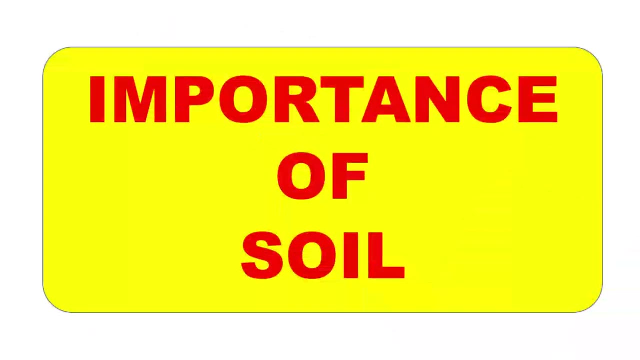 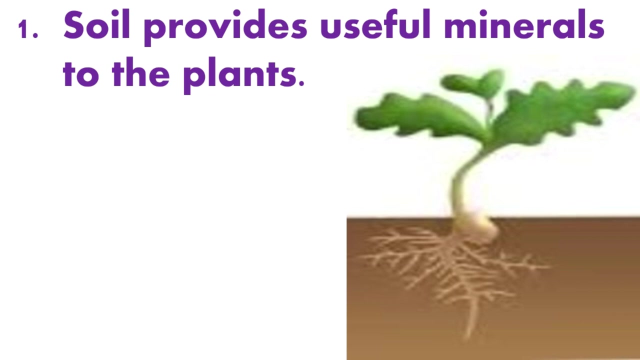 And the third one is bad rock. The bottom most layer is the bad rock And it is quite deep inside the earth And contains large species of rocks. So next topic is importance of soil. So soil is very important for the growth of plants. 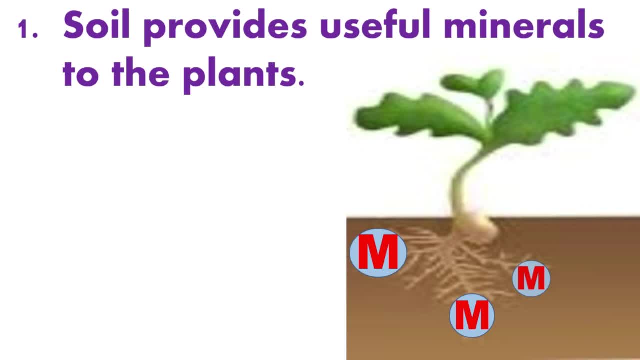 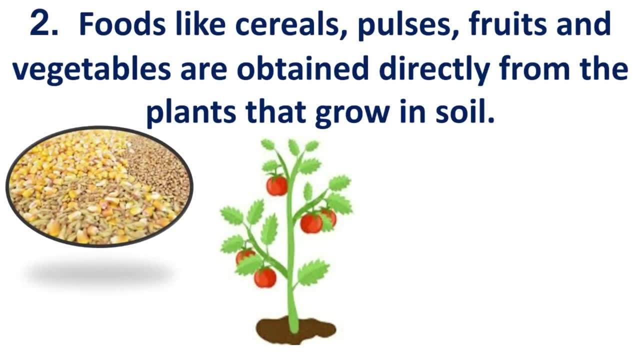 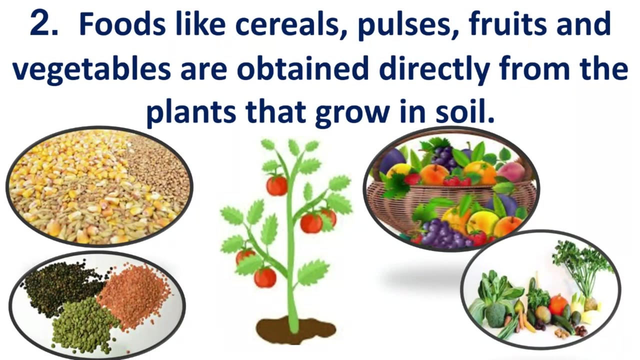 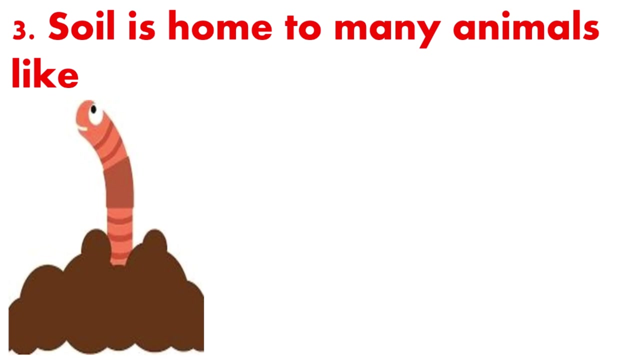 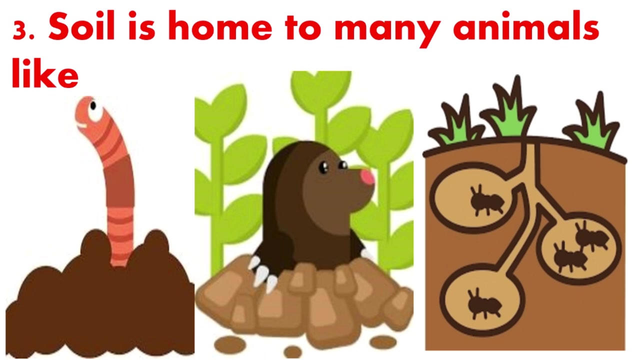 It gives them water and minerals. Minerals are like food for plants. The second one is foods like cereals, pulses, fruits and vegetables are obtained directly from the plants that grow in soil. The third one is soil provides home to many animals like earthworms, moles, ants, rabbits, snakes, etc. 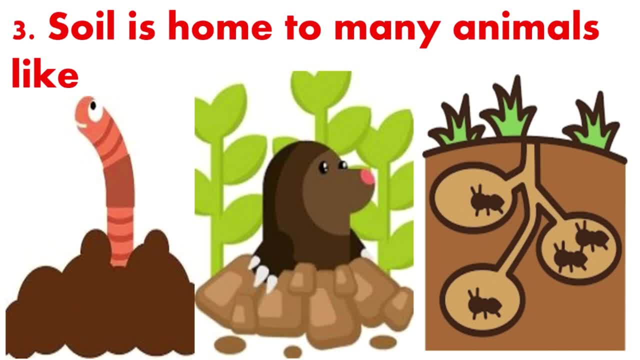 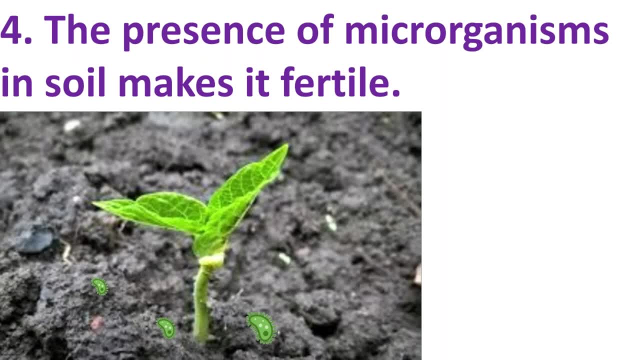 These animals lives in their own way And improves the nature of the soil. The fourth one is the presence of microorganisms in the soil makes the soil fertile. Fertile means soil that is capable of producing healthy crops. Dear children, do you know an interesting fact: that a special bacteria named rhizobium lives in the roots of liguminous plants? 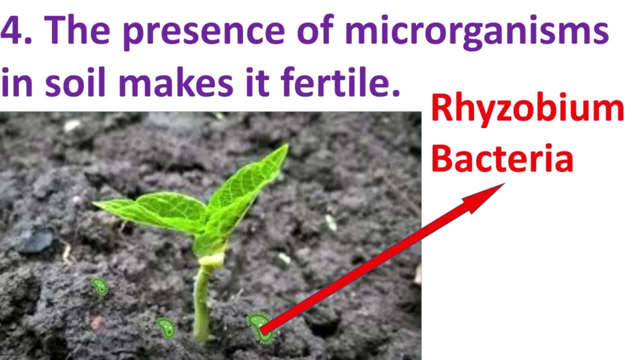 An example of liguminous plants are peas, gram and beans, And you all know that there are many gases present in the air, And nitrogen is also one of the gases which is absorbed by the plants, And most of the nitrogen is taken up as a nitrate. 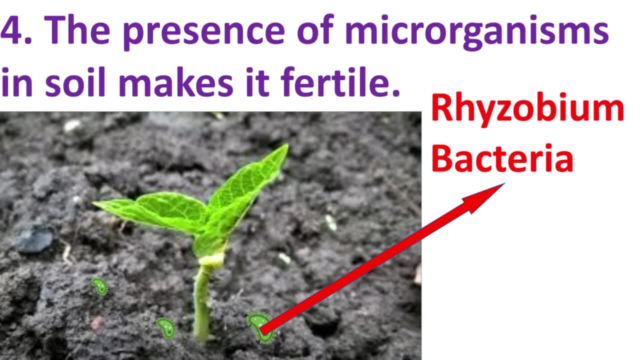 And nitrate moves directly towards the plants roots as they absorb water. So what is the role of rhizobium bacteria? Rhizobium bacteria converts the nitrogen into nitrate. So this was all about soil, And now you know that soil takes millions of years to form. 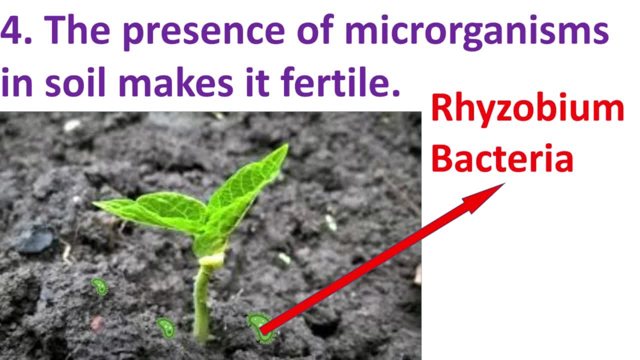 And what is the importance of soil? Hence it is our duty to protect the soil, And soil can be protected by planting more and more trees. So, dear children, if you like this video, please like it, share it, and don't forget to subscribe my channel. 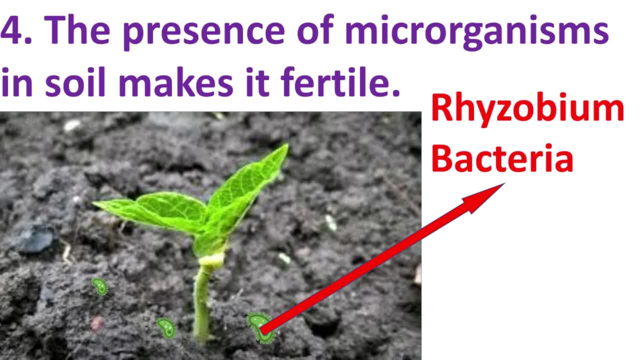 And also hit the bell icon so that you can get the notification of my upcoming videos. Till then, stay safe and have a nice day.